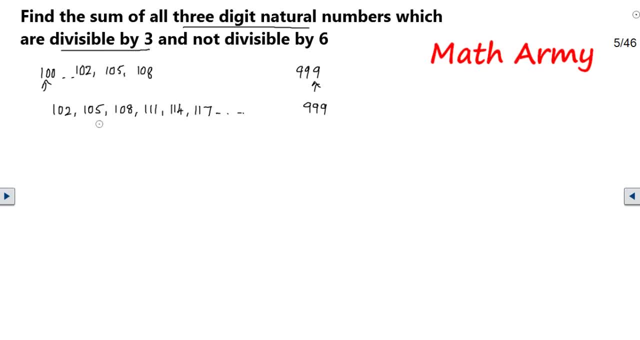 numbers which are divisible by three. okay, now again let us revisit the question. what they are saying? not divisible by six. now is 102 divisible by six. just check. yes, so 102 is not a part of our arithmetic progression. so just put a cross mark. and now is 105 divisible by six? no, so 105 is part of our arithmetic progression. even 108 is divisible. 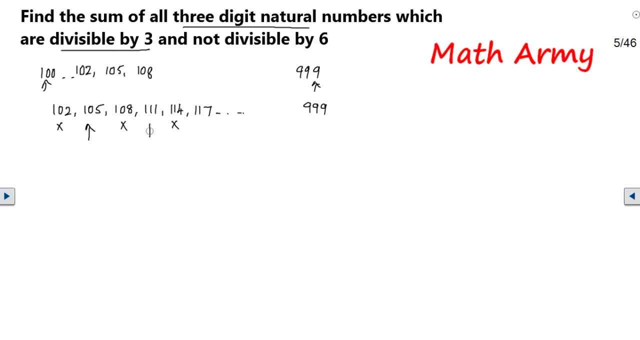 by six. 114 is also, so every second number is divisible, which is divisible by three but not divisible by 6. you know, that is our understanding. so therefore, the arithmetic progression that is going to be formed, which is divisible by 3 but not divisible by 6, are going to be: 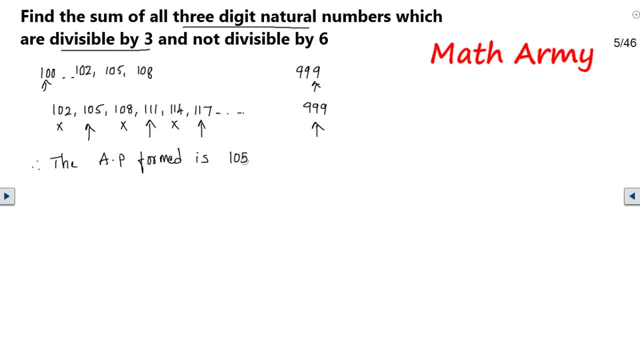 105, 111, 117, so on up to 999. okay, i believe i explained enough about the forming of the arithmetic progression, so from here on, anybody can do it. so 105 is going to be our first number, which is a, and the common difference is a2 minus a1, which is 6, and the 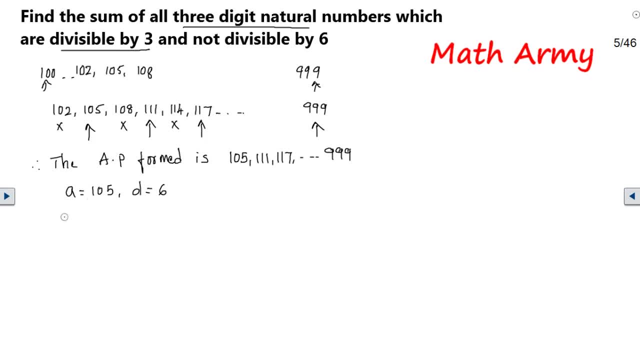 last number, an, is equal to 999, and what these people are asking to find, the sum, and what is formula of the sum? sn is equal to n by 2 multiplied with 2a, plus n, minus 1 multiplied with d. so till here it is fine. 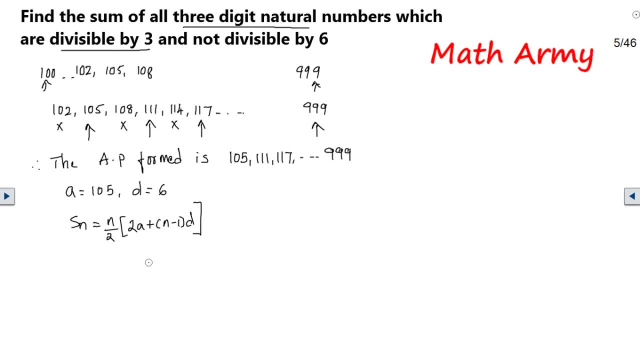 so we have a value, we have d value, but we do not have n value to proceed further, right? so what to do? we need to find the nth number first, n. so what is the formula? an is equal to a plus n minus 1 multiplied with d, and a of n value is 999, which is the last digit right. 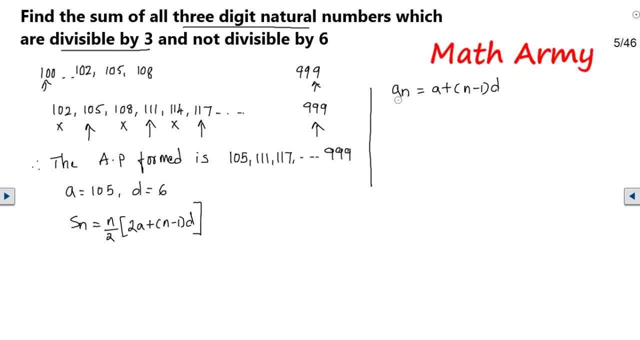 okay, right, 999 is equal to what is the a value, 105 and n value, we don't know. so write n minus 1, as is, and d value is 6. now write 999 now equal to 105 plus 6. multiplied with n minus 1 is 6 and minus 6. 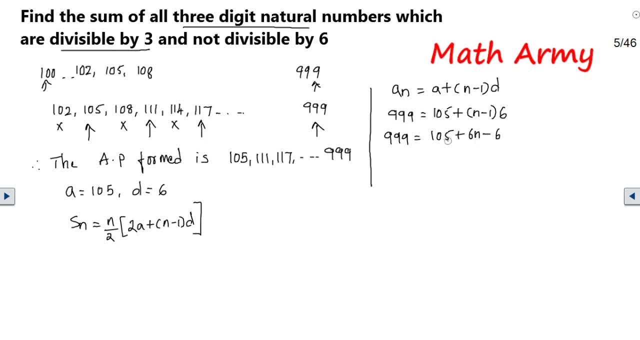 now 105 minus 6 is 99. guys, now 99. bring it to the left hand side, it becomes minus 99. okay, so therefore, 6n is equal to 900. okay, therefore, n is equal to 900. therefore, n is equal to 900 divided by 6, which is going to be 150. 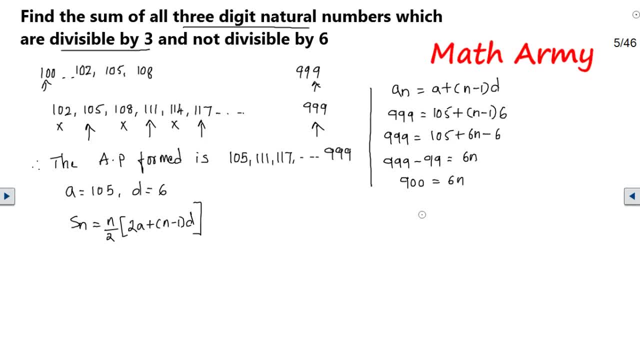 right. just, you know, do a random calculation. six ones are six, okay, three or six fives are, so 150. so i'm just doing a. you know math here. so six divides one, fifty nine hundred in 150 times. so that's it for this video. thank you for watching and i will see you in the next video. bye, bye. 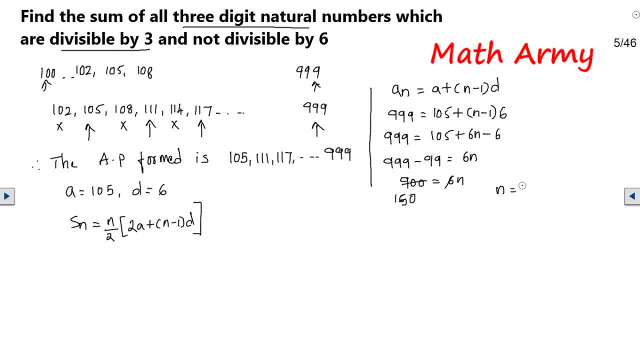 now, once you got the n value, which is 150. now let us come back to the sum problem. okay, now s of n. right, as is now, n by 2 is nothing but 150 divided by 2, multiplied with 2, multiplied with a, so 2 multiplied with size 105. 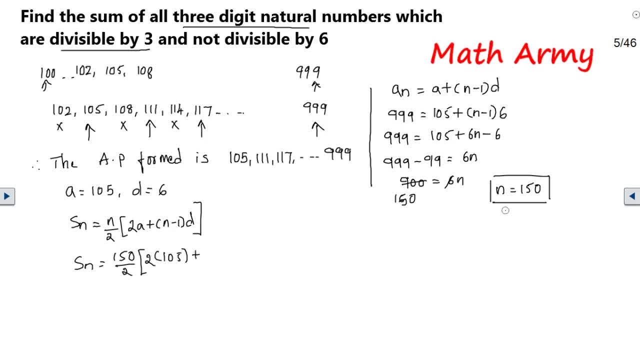 x as 50 plus 1.. what is x, 1, 150 minus 1, and the value is 6. okay now, 150 divided by 2 is 75, and 105 multiplied with 2 is 210, and 150 minus 1 is 149. 149 multiplied with 6 is going to be: